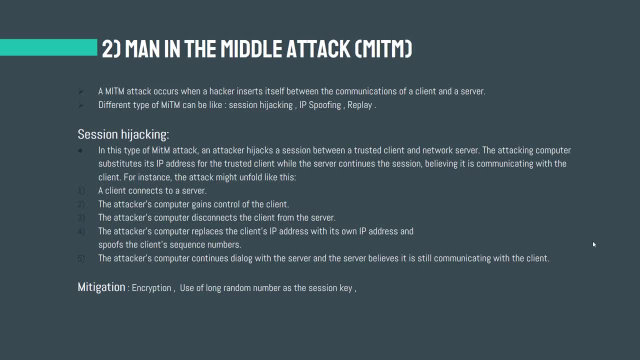 For instance, the attack might unfold like this: A client connects to the server. The attacker's computer gains control of the client. The attacker's computer disconnects the client from the server. The attacker's computer replaces the client's IP address with its own IP address. 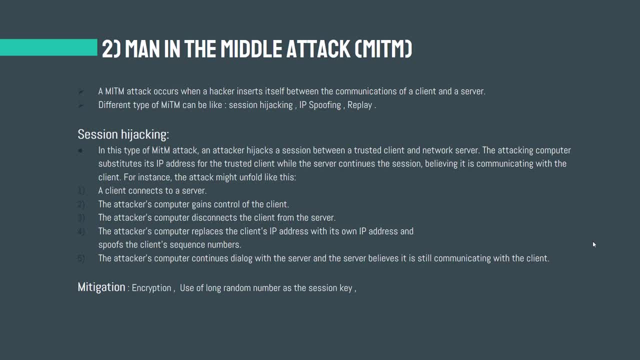 And this spoofs the client's sequence number And number five. the attacker's computer continues dialogue with the server And the server believes it is still communicating with the client. The mitigation mechanism for the session hijacking can be encryption and use of a long number. 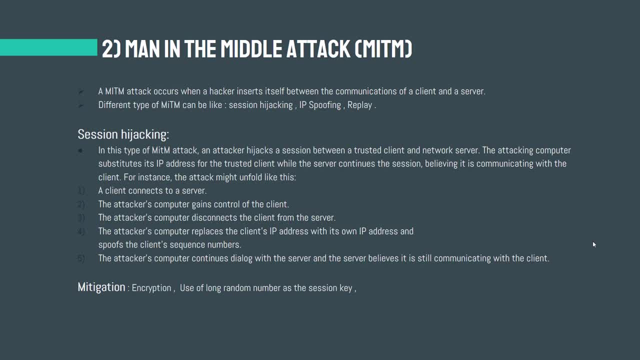 as the session key, Encryption of the data traffic passed between the parties by using SSL or TLS, In particular, the session key. This technique is widely relied upon by web-based banks and other e-commerce services, because it completely prevents sniffing style attacks. 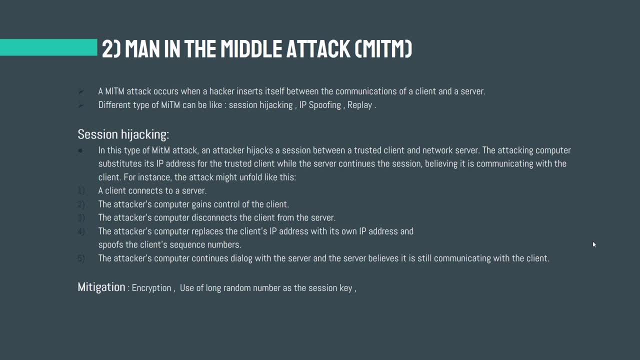 However, it could still be possible to perform some other kind of session hijacking. The second solution for the mitigation of session hijacking is use of a long random number or string as the session key. This reduces the risk of the attacker's data traffic. 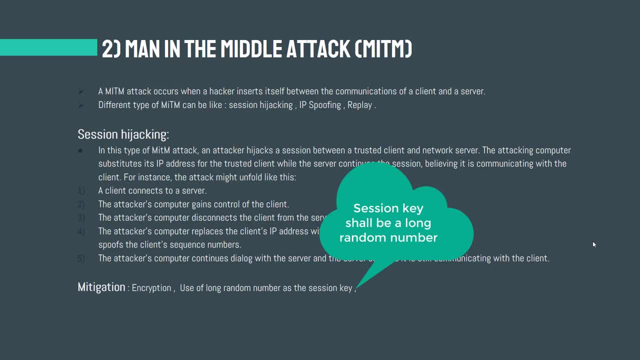 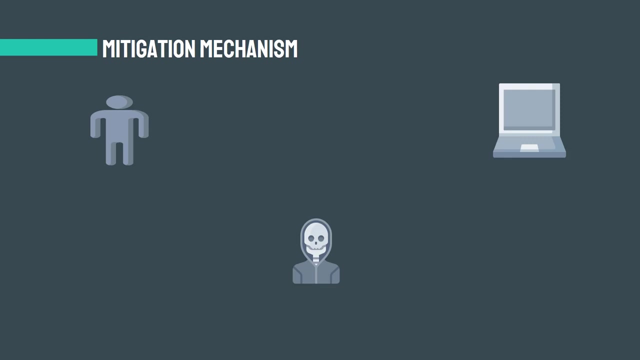 The risk that an attacker could simply guess a valid session key through trial and error or brute force attacks. Okay, Let me show you one very simple simulation from the session hijacking. The client sends a request to the server with the user X and the password 1234, but one. 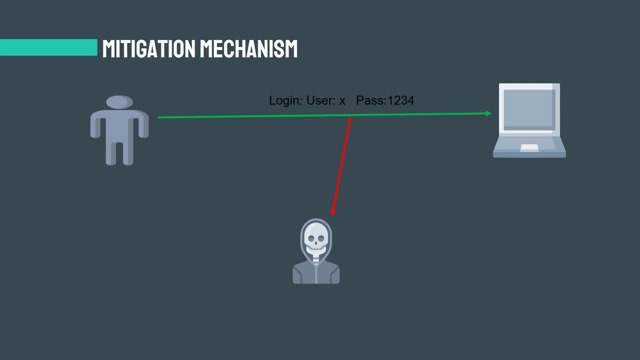 malicious hacker is here, The user X and the password 1234.. But one malicious hacker is here, The unauthorized person is here and he gets all of this information When the server is passing the session ID XYZ to the client- again the unauthorized. 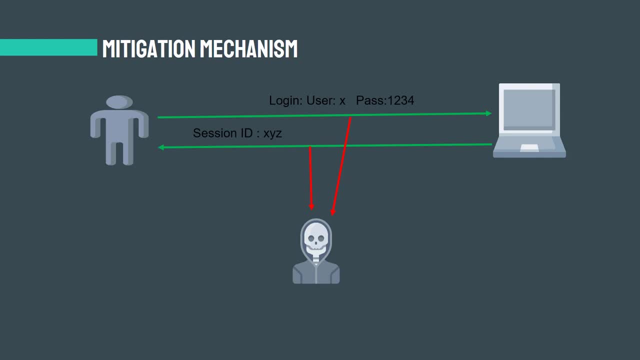 person can read this information and after that, using the session ID, the attacker can continue its communication with the server and in this way, server believes that it is communicating with the right client. Okay, For the next type of the man-in-the-middle attack, we have the IPS spoofing. 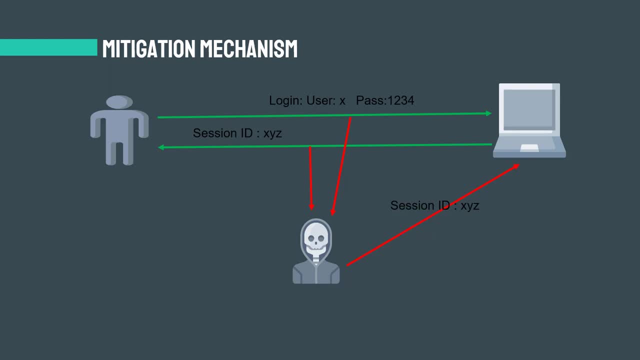 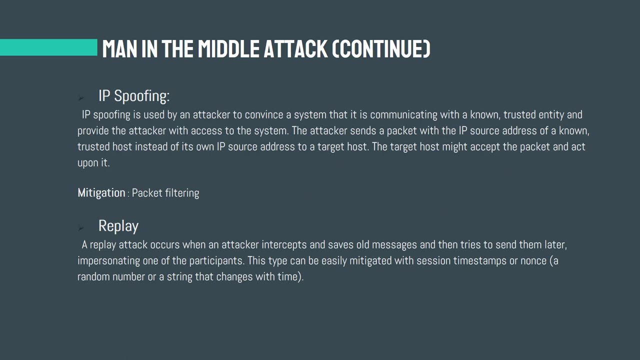 IPS spoofing is used by an attacker to convince a system that it is communicating with a known trusted entity and provide the attacker with access to the system. The attacker sends a packet with the IP source address of a known trusted host, instead of its own IP source address, to a target host. 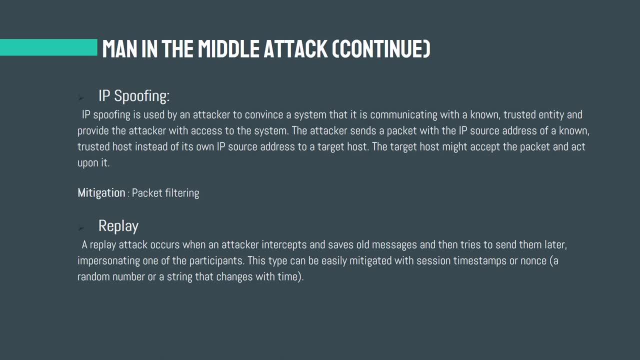 The target host might accept the packet and act upon it. Actually, the mitigation mechanism is very simple. It's packet filtering. Packet filtering because it's one defense against IPS spoofing attacks. The gateway to a network usually performs ingress filtering, which is blocking of packets. 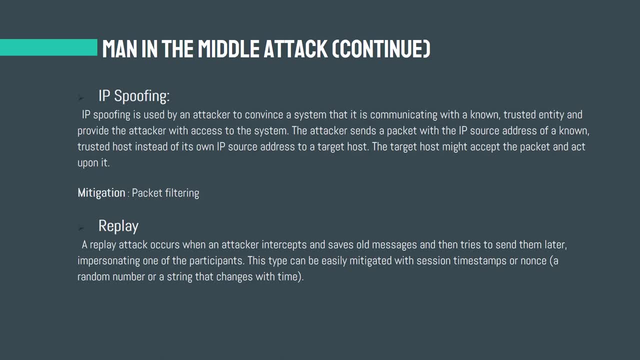 from outside the network with a source address inside the network. This prevents an outside attacker spoofing the address of a network. Ideally, the gateway would also perform ingress filtering on outgoing packets, which is blocking of packets from inside the network with a source address that is not inside. 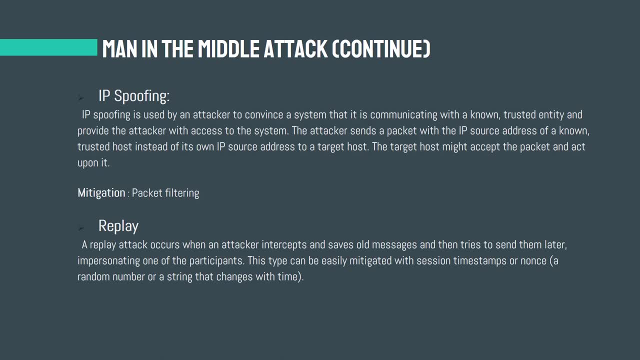 This prevents an attacker within the network performing filtering from launching IPS spoofing attacks against external machines. It is also recommended to design a network protocols and services So that they do not rely on the source IP address for authentication- Another type of the man-in-the-middle attack that maybe you have listened a lot about that. 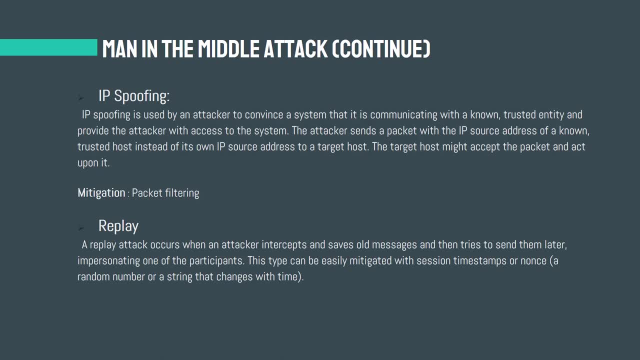 is a replay attack. A replay attack occurs when an attacker intercepts and saves all the messages and then tries to send them later, impersonating one of the participants. This type can be easily mitigating with session timestamps or NAMs. The NAMs is a random number or a string that 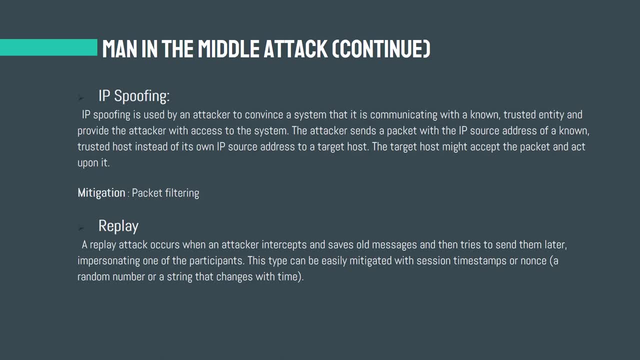 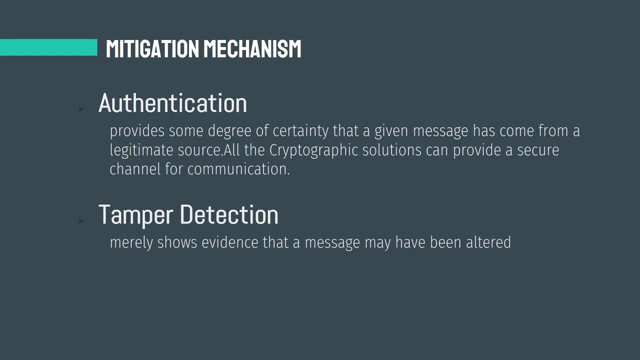 changes with time. Okay, now we have a little bit familiarity with the man-in-the-middle attack and some sort of the mitigation mechanism that I provide for you. In general, the mitigation mechanism for the man-in-the-middle attack can be categorized in two subcategories: authentication and tamper detection. 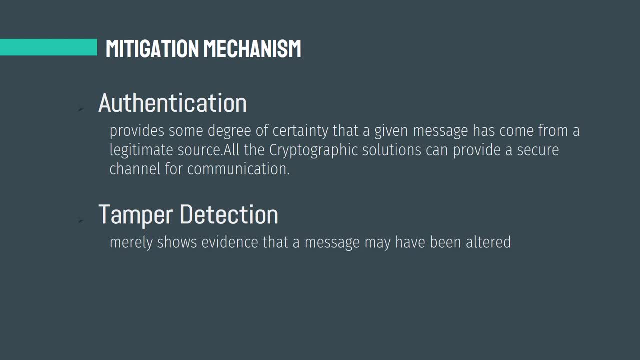 Authentication provides some degree of certainty that a given message is being sent to the attacker. Authentication provides some degree of certainty that a given message is being sent to the attacker. The message has come from a legitimate source. For the authentication we have a lot of techniques, like some sort of a digital certificate, and